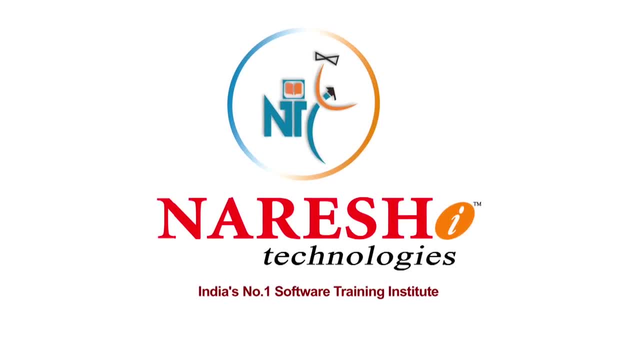 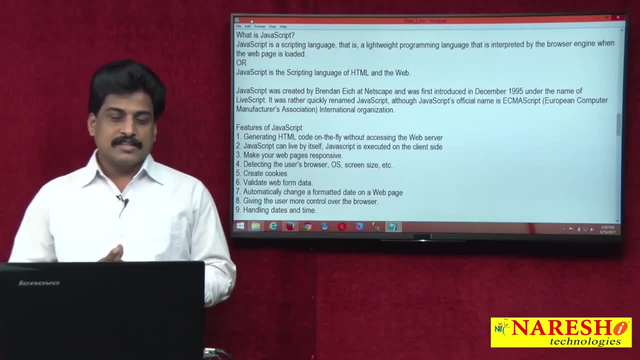 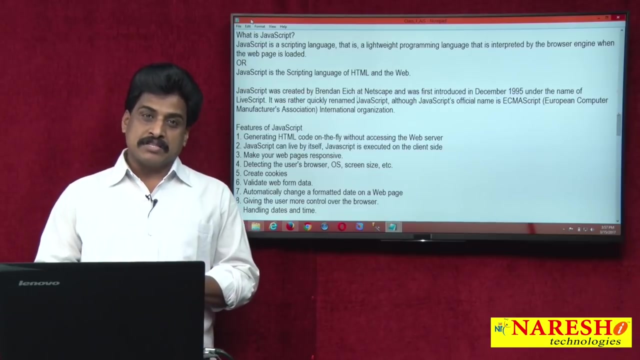 Hi guys, welcome to Narayansha Technologies. This is Subbarajo. In this session we can view JavaScript, introductory part. What is JavaScript? JavaScript related features. who developed that and what is exact name of the JavaScript? the syntax of the JavaScript JavaScript is: 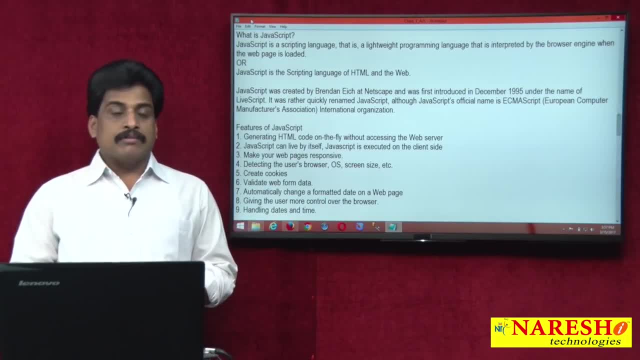 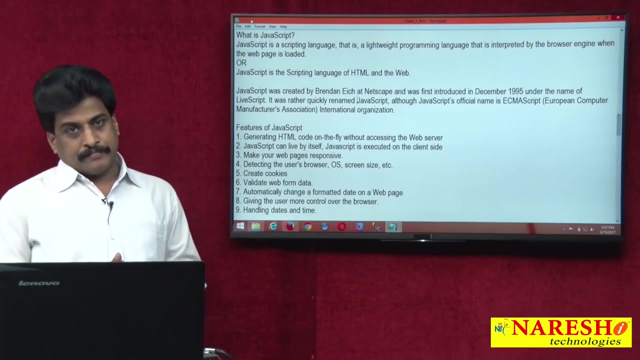 weekly typed programming. JavaScript. originally original name is LiveScript. We are calling as LiveScript. It is completely developed based on C language syntaxes. LiveScript developed in Netscape Corporation in 1990s, In 1995, Braden Itch- there is a popular scientist. 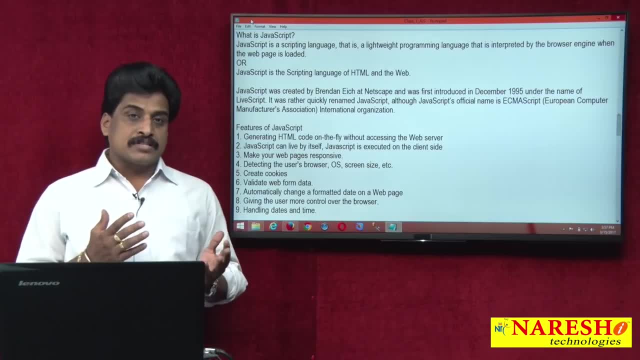 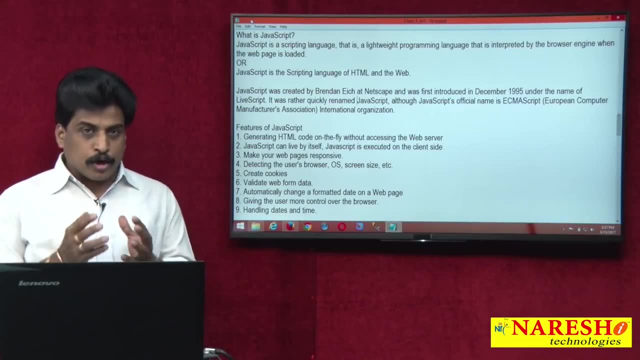 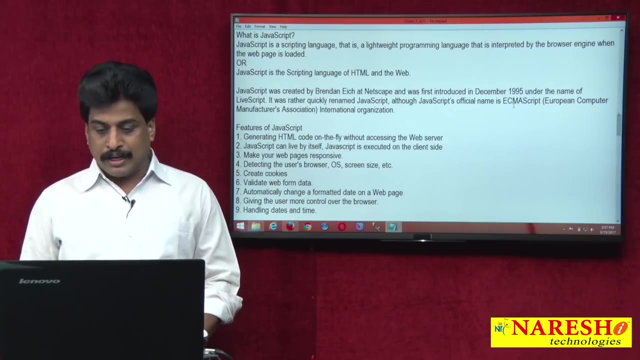 from Netscape Corporation. He renamed LiveScript to JavaScript, So if you are going to view JavaScript syntax, it is very close to C languages, C language syntaxes. JavaScript official name is ECMAScript. We are calling as ECMA- European Computer Manufacturers Association. It is. 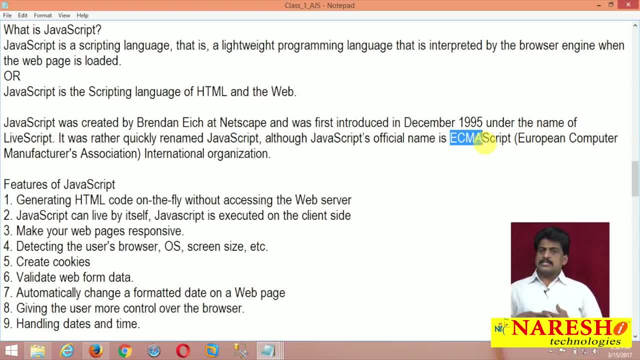 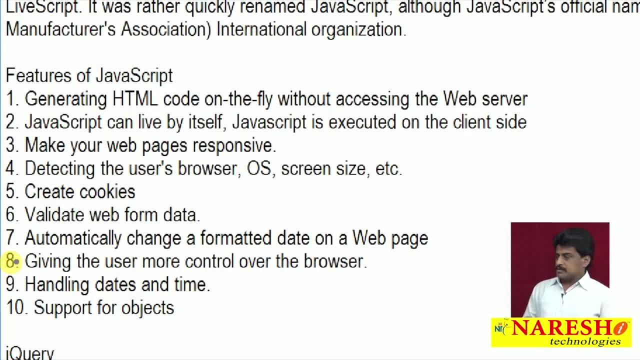 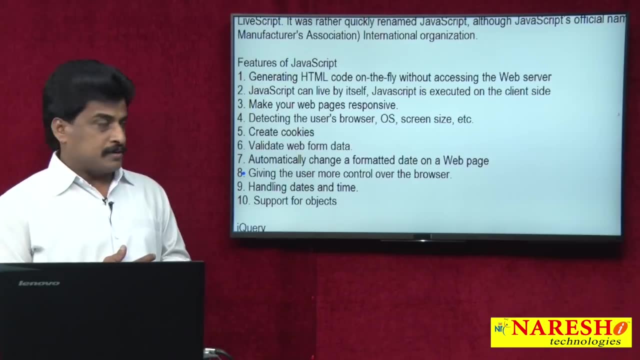 one kind of international organization. There are the several features of JS Already. in last video session I spoke about script advantages. Same almost all here. Completely client side. any information you can track with the help of JS Generating HTML code, HTML CSS. 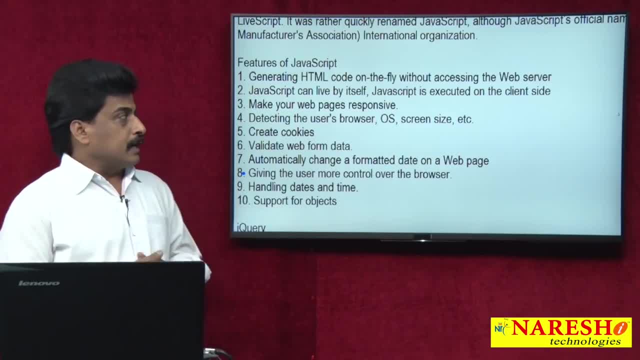 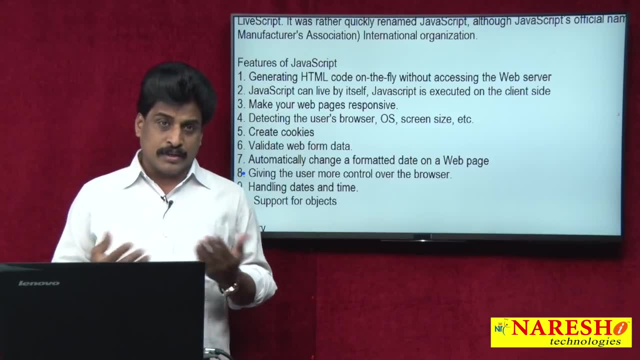 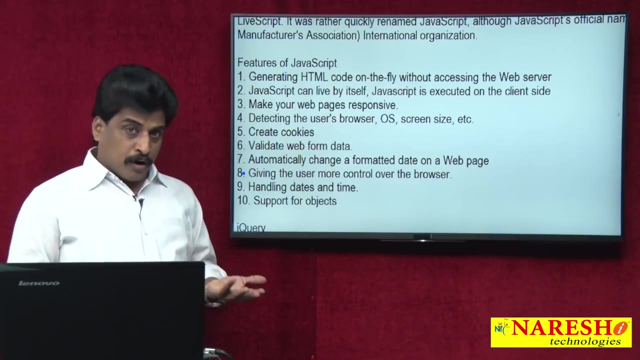 itself static With the help of JavaScript we are making dynamic. JavaScript can live by itself. JavaScript is executed on the client side. I think already I said that one. It is a browser level, It is a web level client. Make your web pages responsive In the sense dynamic here Responsive. 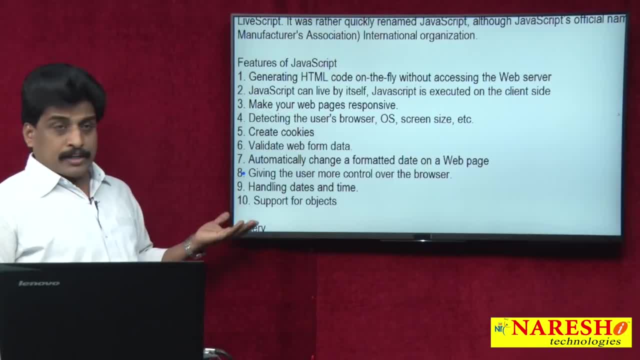 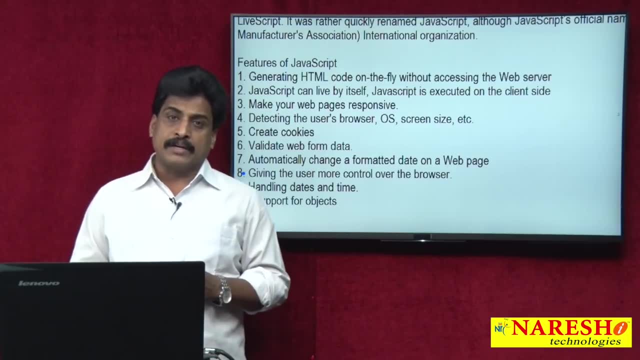 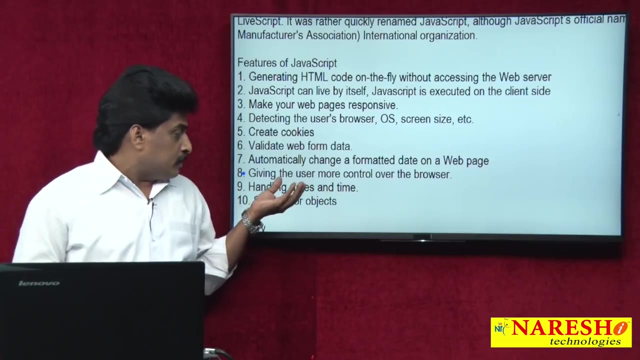 in the sense not bootstrap kind of features. Create cookies. Validated applications, For example HTML forms are there. Text boxes, password, check box, radio button Like this. You want to validate those. You can use JavaScript And giving the user more control over the. 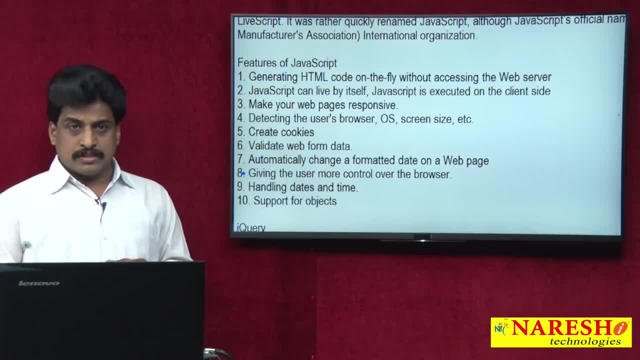 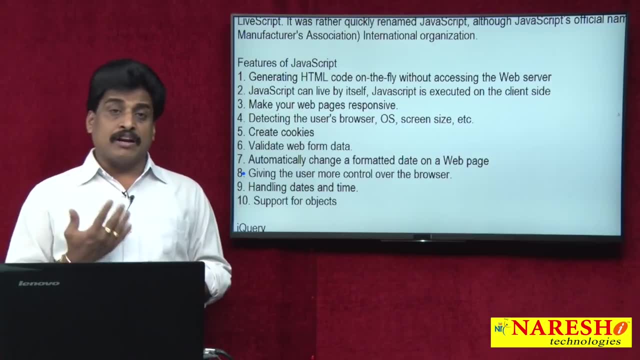 browser. Yes, you want to apply. the more controls Means any action you need to perform on the web page. JavaScript is providing to us that, Supporting for objects. there are several objects available. JavaScript is object-based programming, Object-oriented programming also. 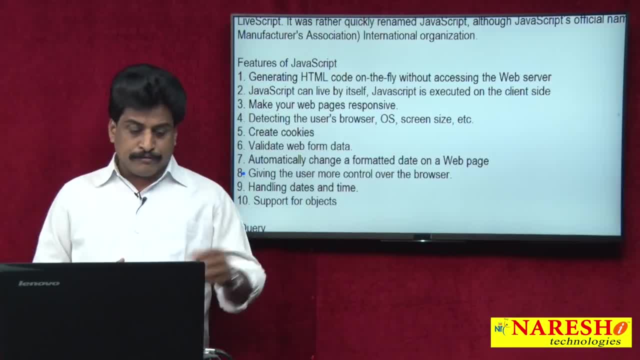 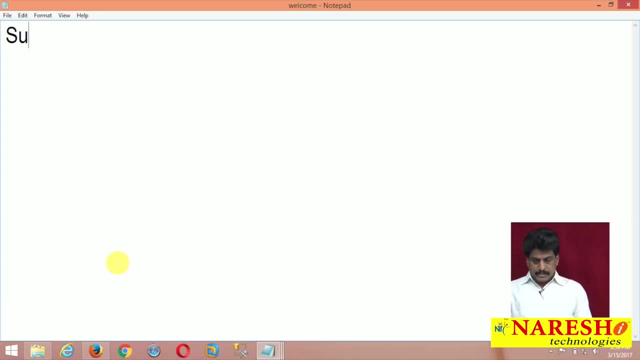 In upcoming days we can see that one practically. So these are the several features of JavaScript. Now we'll go to practically syntax. is what exactly JavaScript? Let me write syntax. And once we are going to JavaScript level, script tag type is equal to text or JavaScript language equal to JavaScript. 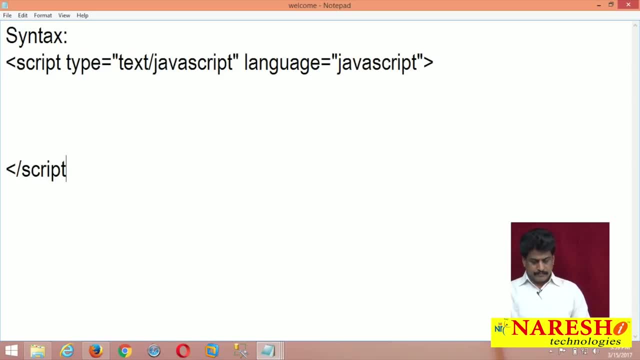 And several statements. you can write scripts, statements, Now statements. Almost all these are the things existed here Now. these all the things existed Now. sometimes we can write like this also, because type is an optional attribute, now Script, This is also perfect. 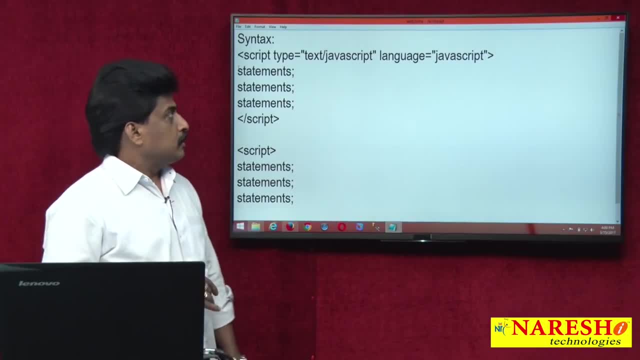 So syntax 1 and syntax 2, both you can observe Here- script is a tag, Type is an attribute, Language is an attribute. This we are calling as MIME types, actually in live environment. So texture, This is what JavaScript is calling as parameter. 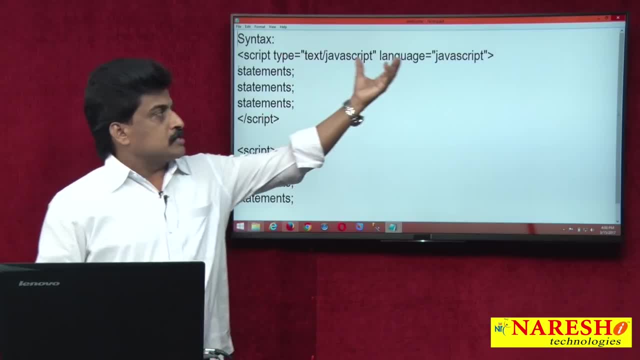 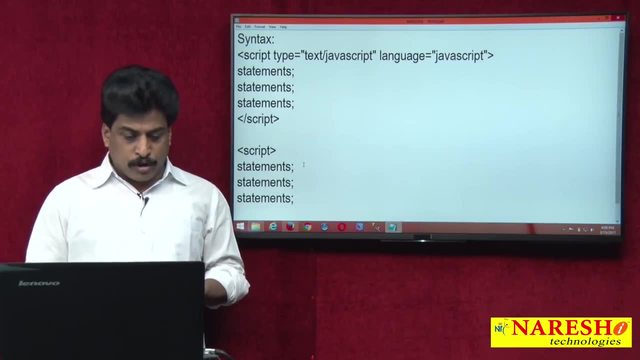 It's not compulsory parameters, So this is an optional. this is an optional. That is the reason. syntax 2: I made very clearly here. It is a weekly type of programming. If you are writing without semi-colon also, it is correct. 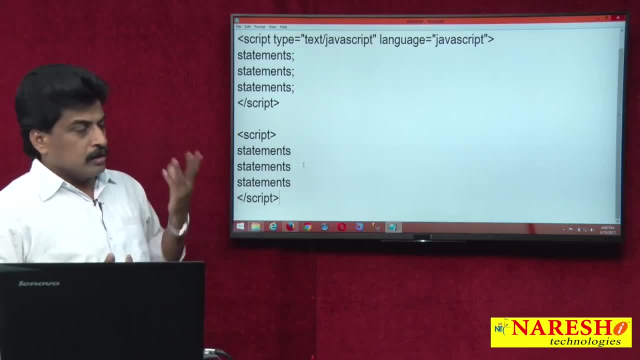 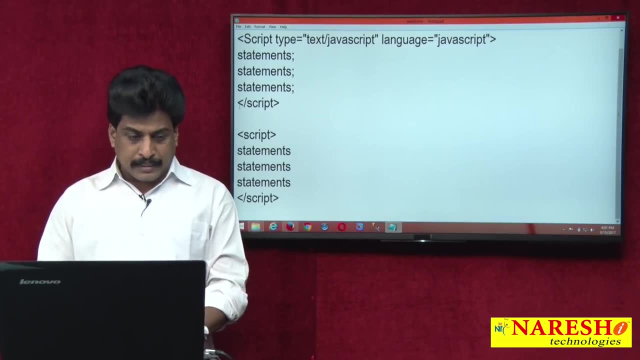 So, syntactically, JavaScript, we can write the above one or below one, Anyone is okay. At the same time, JavaScript is case sensitive, Even though you can write here capital letters, because why you are writing capital letters here means it is a HTML. 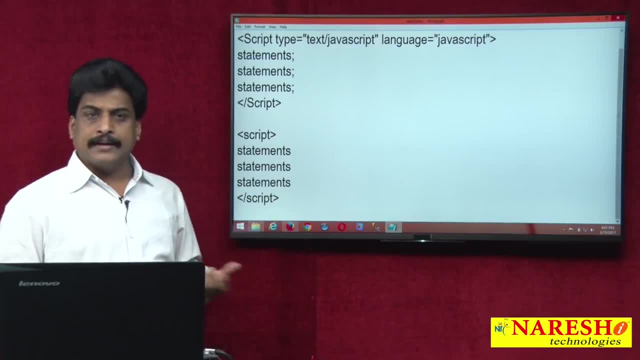 HTML you can write in uppercase, lowercase any case. no problem, Script is not JavaScript. This is the part is JavaScript. This part is HTML. This part is HTML. So HTML can be uppercase as well as lowercase, No issue. So script we can write in uppercase as well as lowercase. 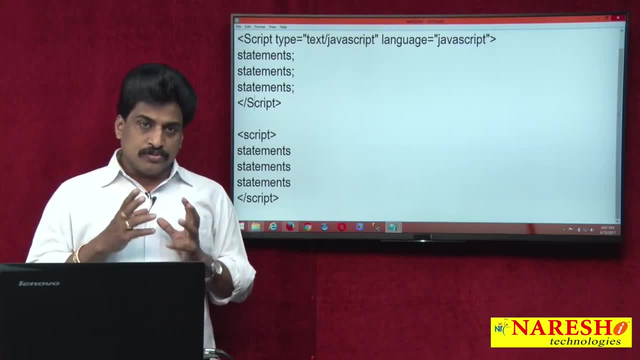 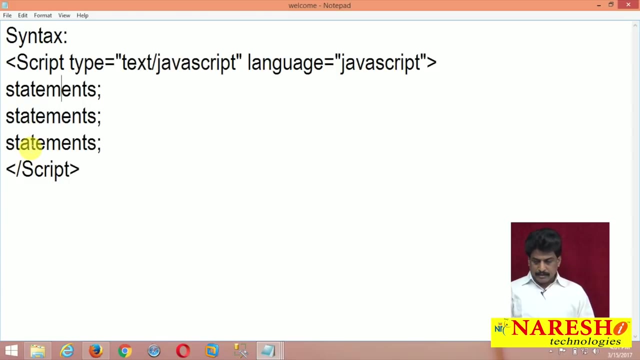 But a script inside. whatever the keywords you are implementing, these keywords must be in lowercase. So this is a small syntax of the JavaScript, And now we can see JavaScript example, Practically how it looks like that. Now come down to JavaScript level. 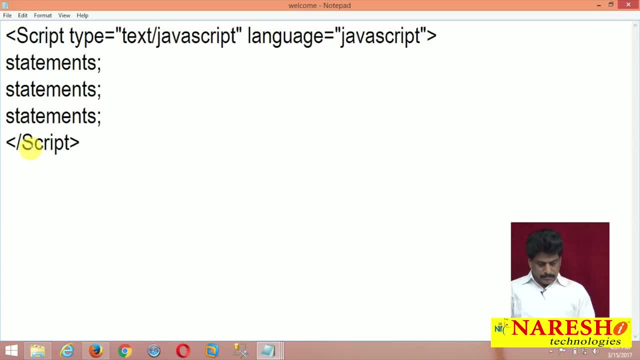 And once you are removing the syntax environment- first script I removed- Now inside I am writing information And within the head section you can write. Within the body section also we can write No issue And if you want, you can maintain doc type also here and doc type HTML. 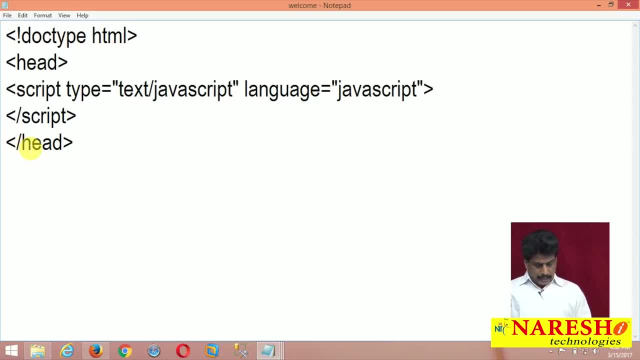 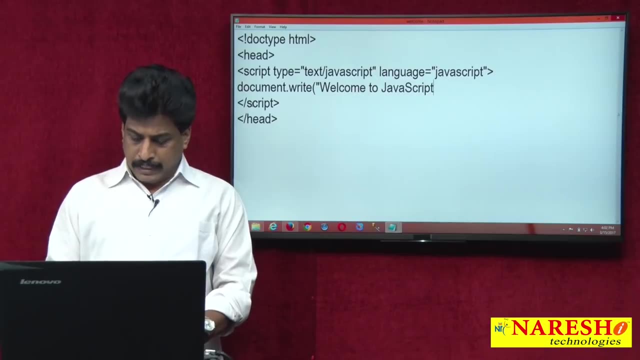 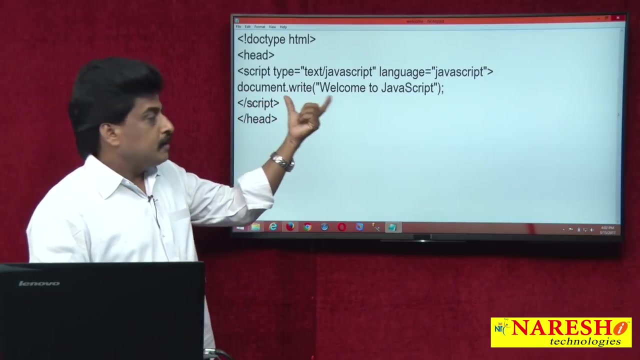 It indicates version information already explained. And now I am calling document dot. document dot. write. welcome to, welcome to JavaScript, welcome to JavaScript. Once I am going to write that it is an object, it is a method, it is what I am going to display on the web page. statement ends not compulsory. 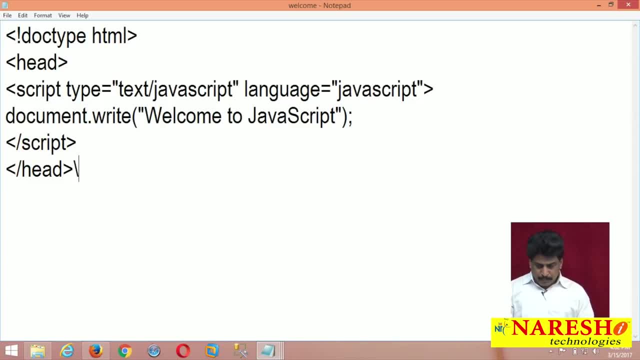 Optional and optional. And right now, this simple program I am saving with save with dot JS extension, correct, But right now I am saving with dot HTML or HTM extension. I am saving like this. I am running fast, Why not dot JS? 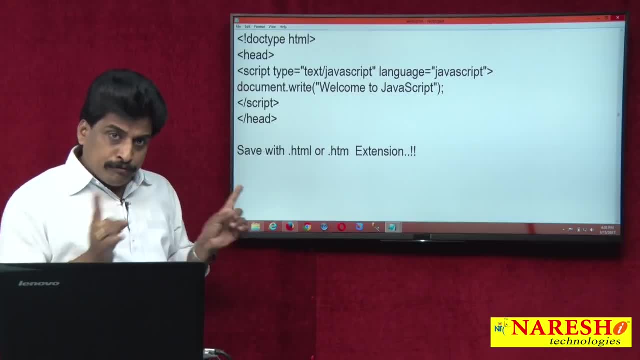 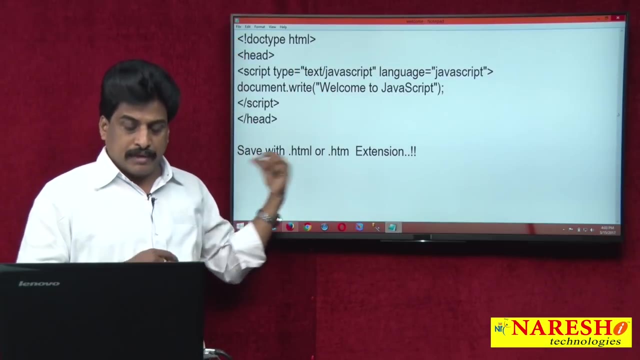 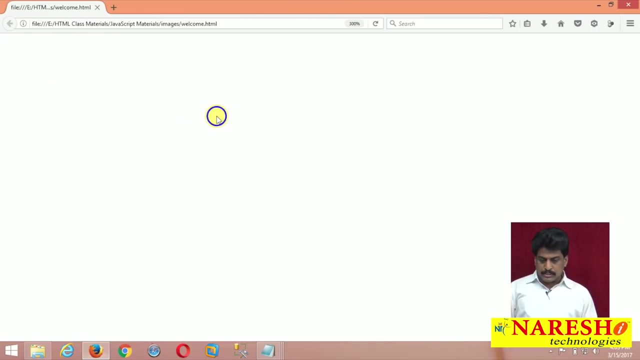 If you ask the question dot. JS file never contains any tag related things. JS file contains only JavaScript, So that means your tags available. that is the reason. HTML. Now, I saved that and I am running with any web browser. Now, just I am going to my browser, right click and refresh that. 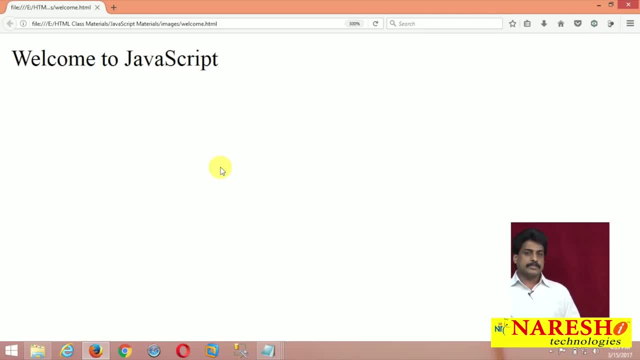 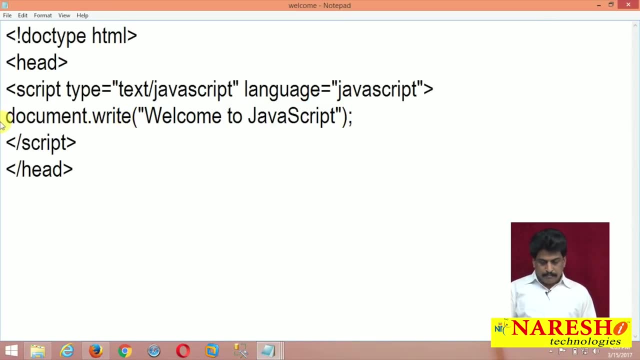 Perfect execution. Welcome to JavaScript. Now this is JavaScript information. simply displayed one statement, For example. I want to display, for example, another statement. like I said, welcome to Naresh technologies, Naresh IT. Once you save that, you can close and open single quotes, right. 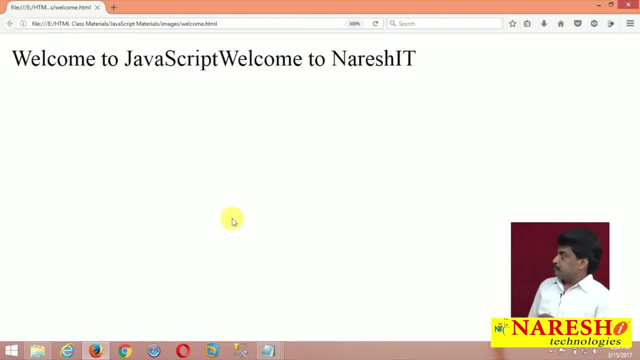 And if you are going to run on your web page, it is running. So welcome to JavaScript, welcome to Naresh IT, But there is no space between that. So whenever you required a space between two lines or two statements, we are using a simple that is called LN. 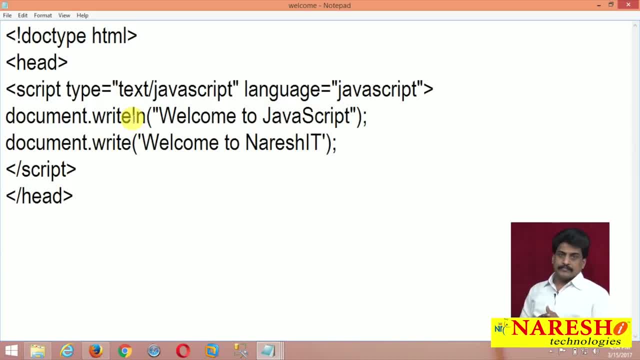 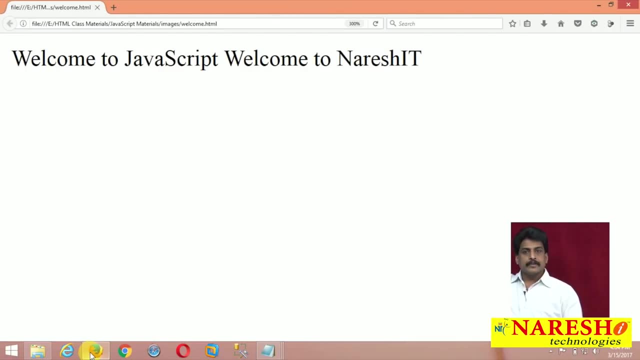 Generally, LN means we are thinking next line. Of course happened that one, But LN is nothing, but it is providing a space between two lines and it is separating now. Observe, Now it is providing or not Perfectly provided. Now you want to display that one in the next line. 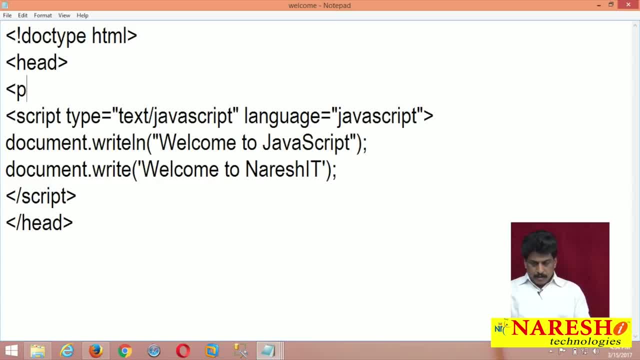 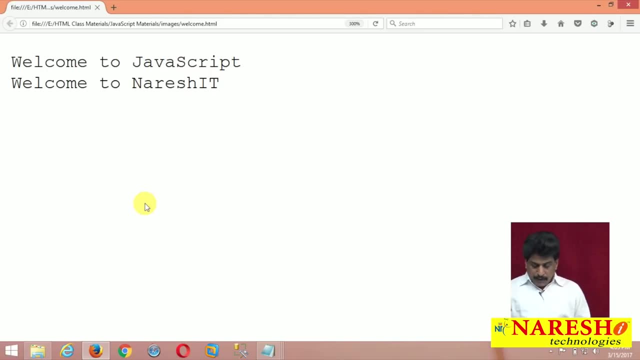 You can use actually PRE-PRE. Why we should use PRE-PRE? And whenever you are using PRE-PRE formatted text, the output displaying in two lines: Welcome to JavaScript. Welcome to Naresh IT. Otherwise you can use. okay, I don't want a pre formatted text. 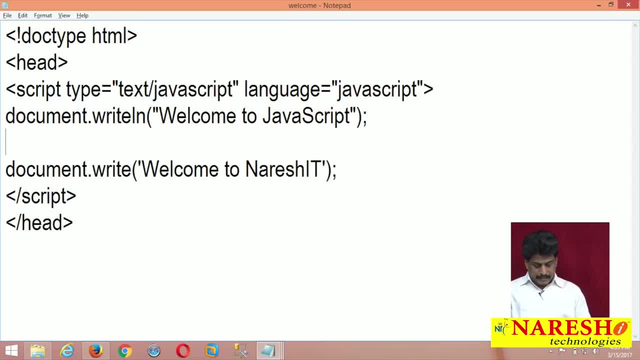 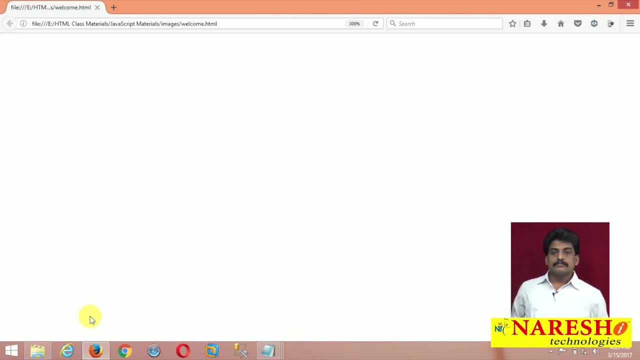 I need, but two lines means You can use a BR tag. Yes, you people are waiting for that. I know that. BR self-close. Now, if I refresh it at a flap, Yes, there is no output. What is the reason behind that? 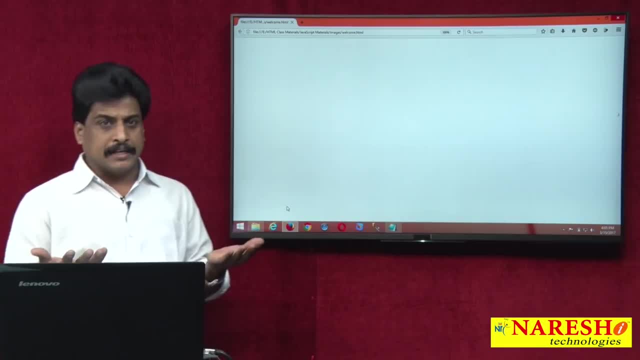 A tag must not be used directly in the script environment area. A tag is different. Tag is from HTML. JavaScript is a programming language. How can you use a markup language inside programming? So there is a syntax rule available. What exactly is the syntax rule? 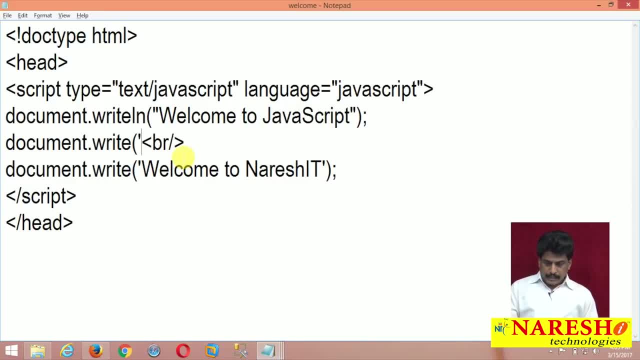 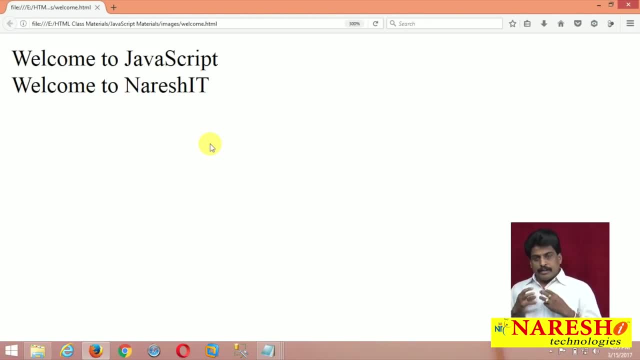 And you must follow document, dot, write and close. Yes, this is a perfect syntax. So whenever you are using a markup language inside JavaScript, you can tell to in JavaScript way Directly. you must not use any tag here, Even though you can come down. 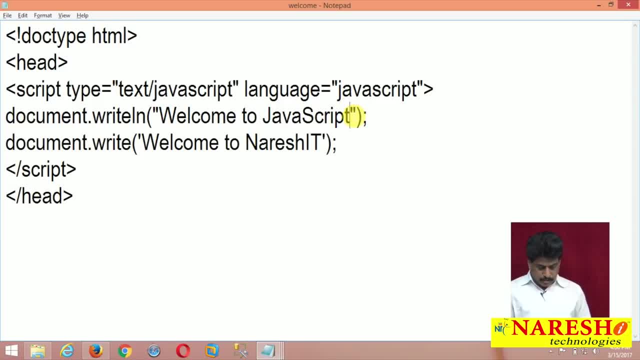 For example: same break you want to use. Yes, you can use like this also, No issue. Yes, refresh Perfect. Where I used correctly observed the area used inside double quotation. I use it. for example: OK, now, I don't want that. 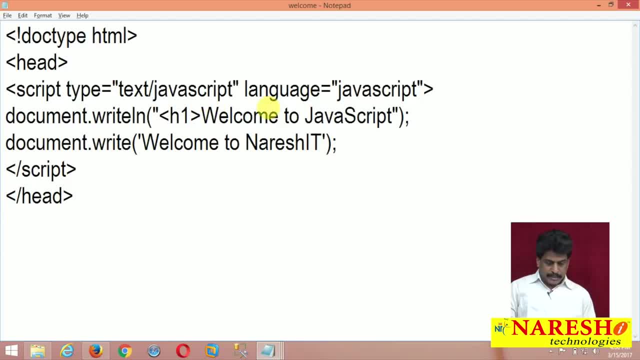 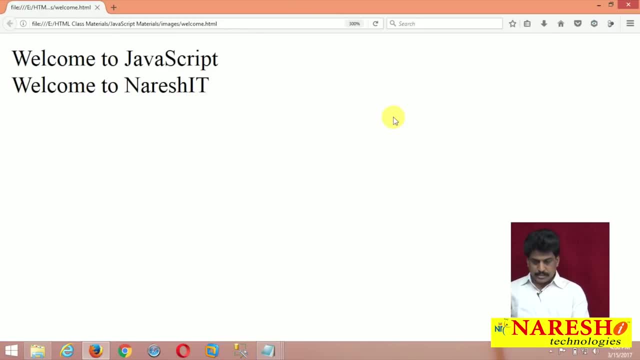 I want to use a tag inside of this. So H1 means you're implementing HTML tags inside scripting. Come on refresh. So I hope you got out to use HTML tags inside the script. So this is the way, simply, effectively, we can implement this. 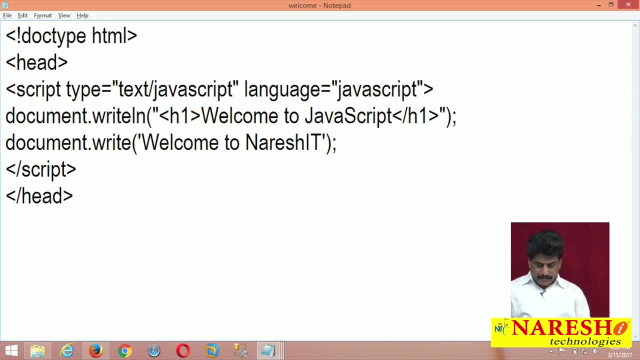 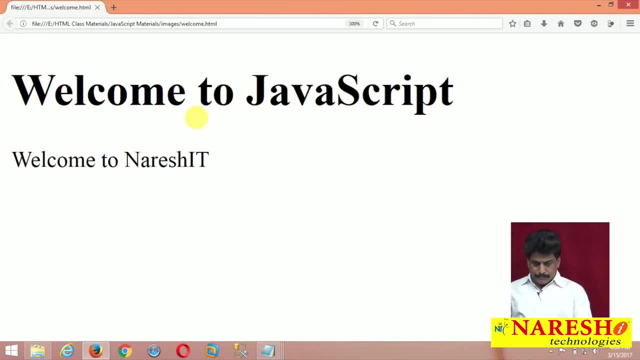 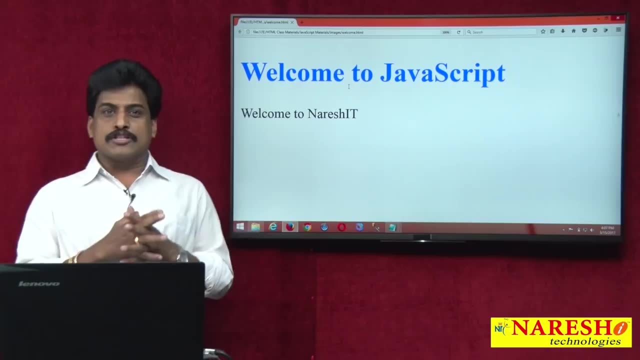 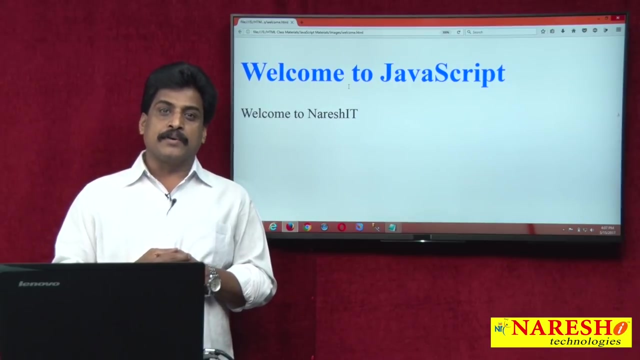 Now I want to apply some kind of styles. even here, Style is equal to color blue symbol. I closer that and I'm refreshing: Perfect. See here: HTML existed, JavaScript existed and style means CSS also used. If you use these three things, what we are calling DHTML, dynamic hypertext markup language. 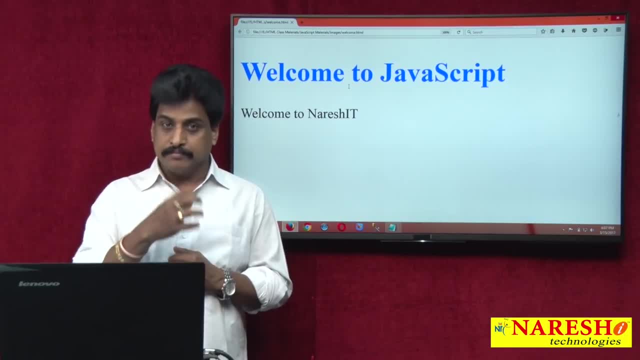 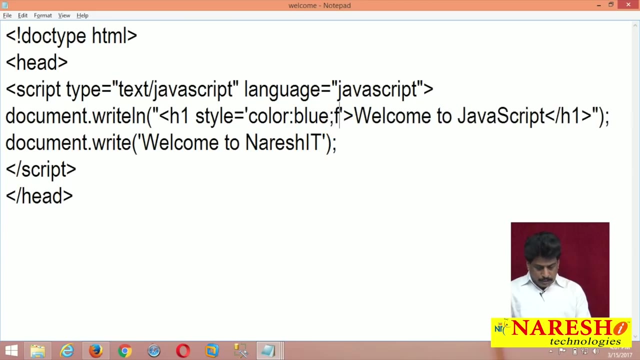 DHTML is One umbrella term where collection of technologies together we are using. Maybe in another video session I'll discuss very clearly about that. Now we can see: for example, I want to apply font family Tahoma and I want to refresh. 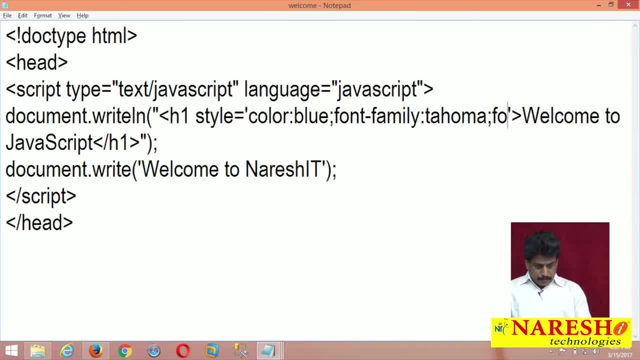 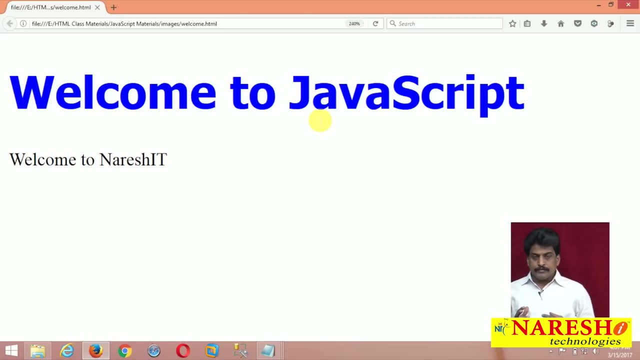 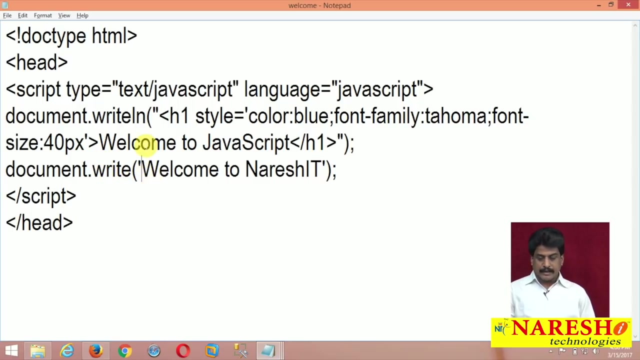 Perfect. Now I want to apply something: font size. I want to decrease, I want to increase. All are possible here With the help of style attribute. I implemented that. Now, if you are going inside a little bit JavaScript here and just the confuse you can see here. 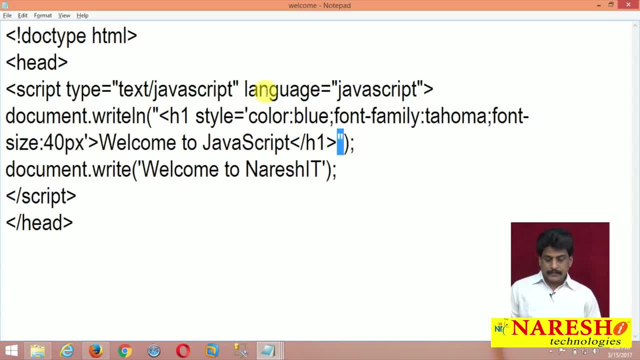 Here double quotation. here double quotation existed. Here single quotation existed. here single quotation existed. Remember, in JavaScript a double quotation inside a single quotation directly we can use Single quotation inside a double quotation directly we can use. But if I use double quotation inside a double quotation, for example, 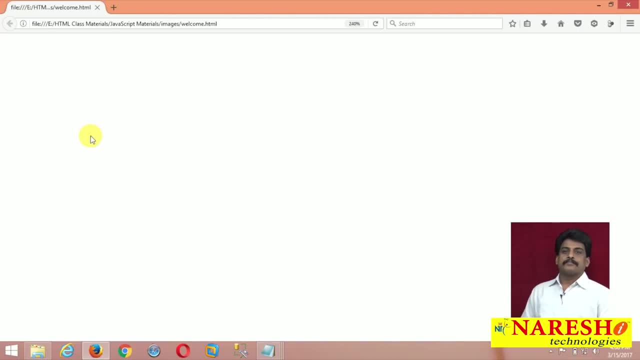 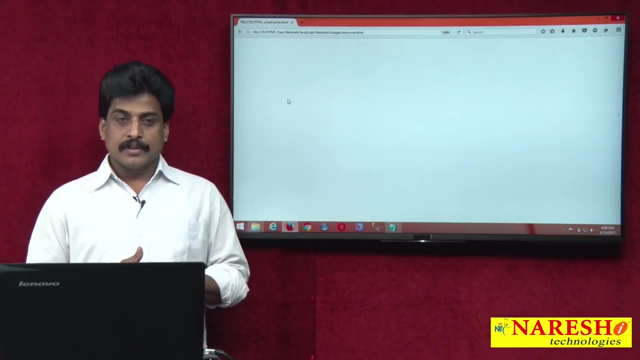 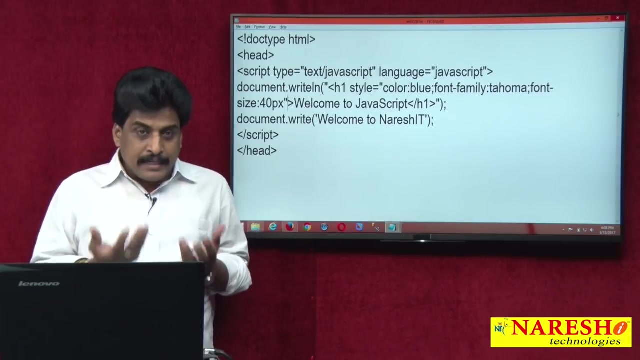 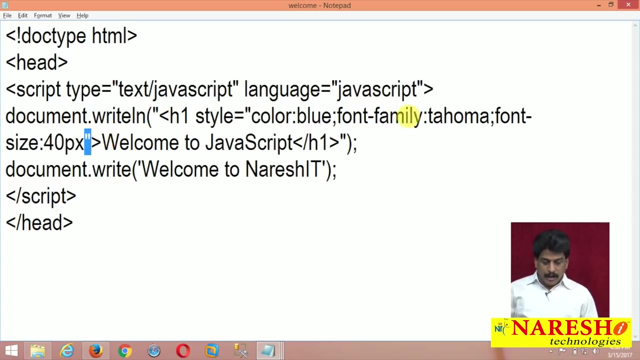 a total example out. Syntactically we made a mistake. Why actually it is a syntactical mistake. Now inside JavaScript interpreter, mechanically it is asking my dear programmer, your string started from here or here or here, Like that it is asking us. it is confusing. 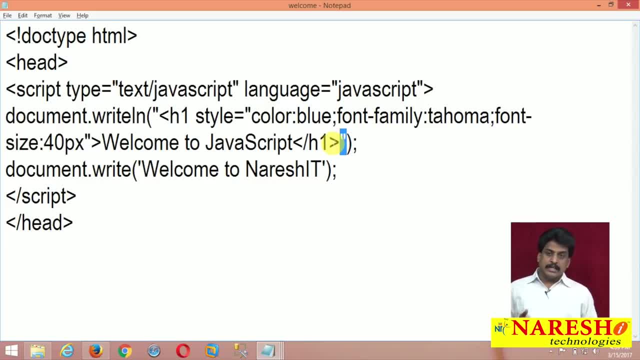 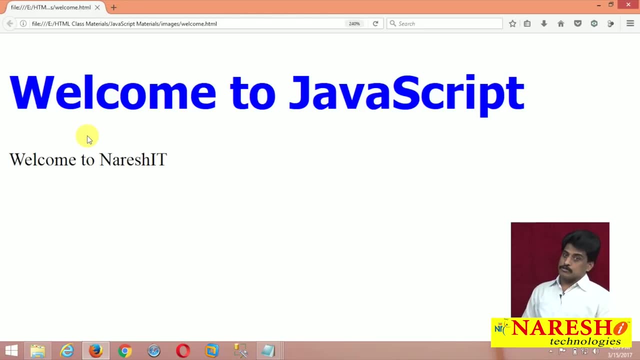 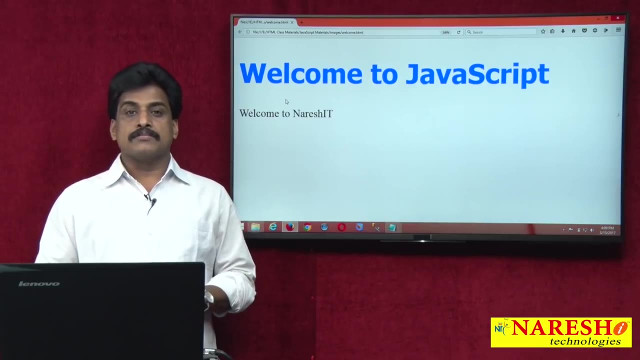 That means double quotation used multiple times. Where is it starting, Where is it ending? Confused In that situation, you must use double inside or single, or you can use here perfect purpose type sequences also. Thank you for watching my videos. For more videos, please log on youtubecom. slash NareshIT.